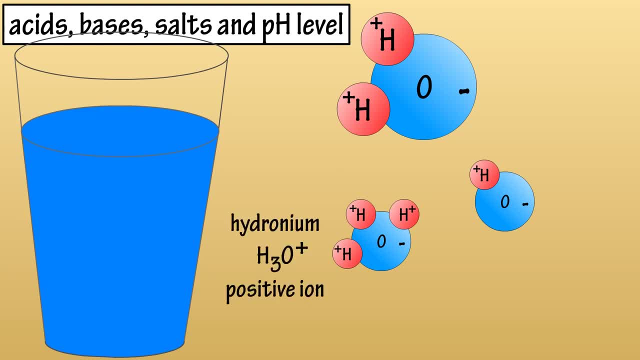 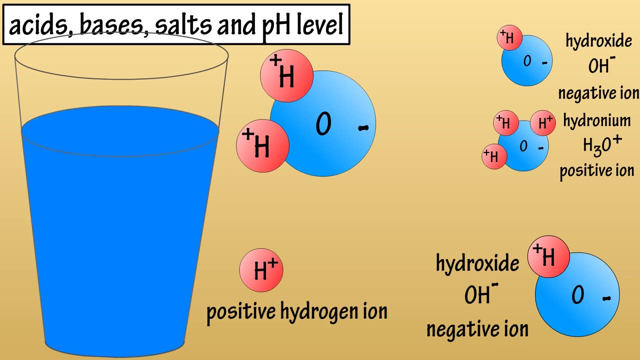 water molecule. So this yields a hydronium or H3O, positive ion and a hydroxide or OH, negative ion. Also, water molecules are called hydrogen atoms. Water molecules continually disassociate to form positive hydrogen ions and negative hydroxide ions. 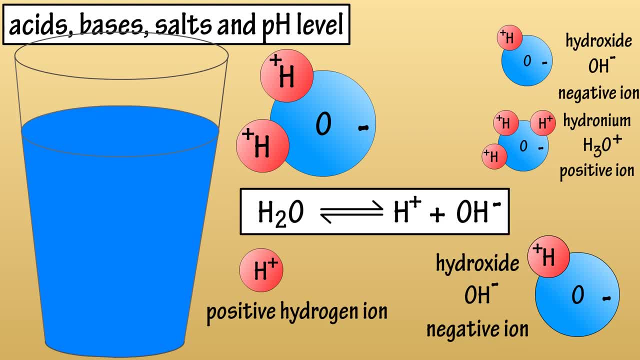 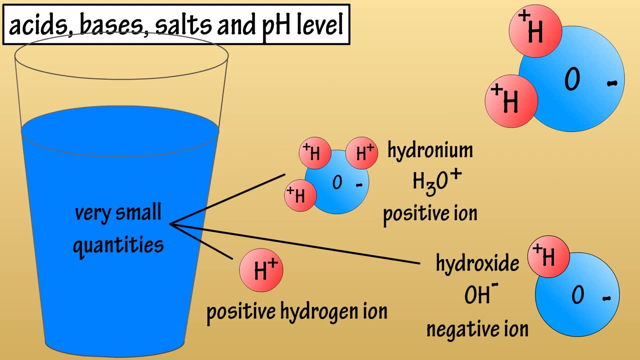 This is a reversible reaction, as noted by the formula H2O double arrow, or reversible reaction: positive hydrogen ion and negative hydroxide ion. The actual amount of these positive H3O or hydrogen ions in water is actually very, very small. To make things easier to understand, we will consider the 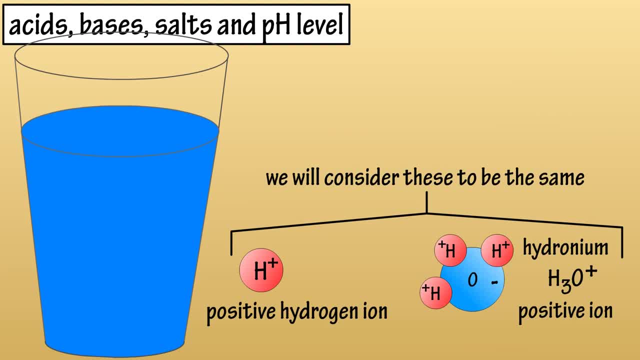 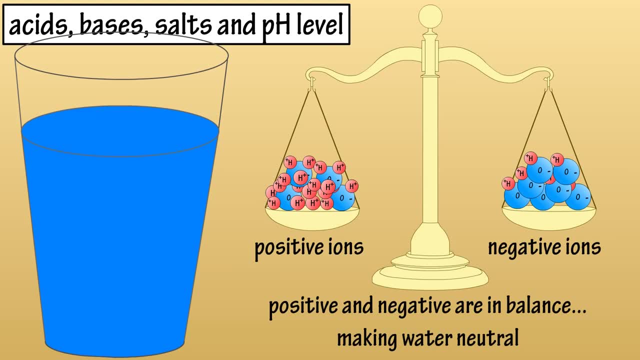 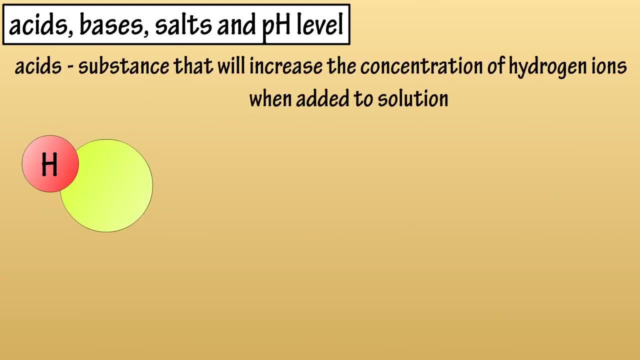 H3O ion and the positive hydrogen ion as one in the same. So in pure water the amount of positive hydrogen ions and negative OH ions is the same. Now for acids. An acid is any substance that, when added to an aqueous solution or water, will release a hydrogen ion or increase the concentration of. 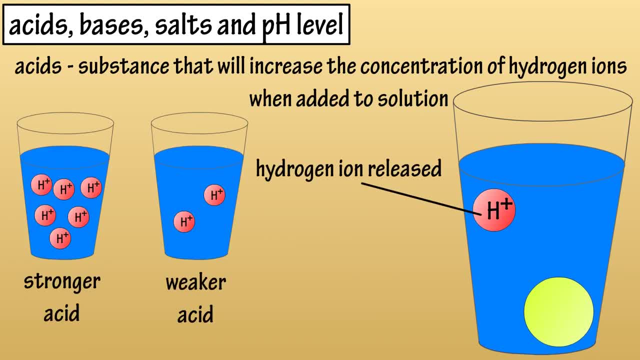 hydrogen ions. So how strong an acid is depends on the amount of hydrogen ions. So the amount of hydrogen ions produced, For instance, hydrochloric acid or HCl, which is a hydrogen atom bonded to a chlorine atom, when added to a solution or water will disassociate or break down into negative. 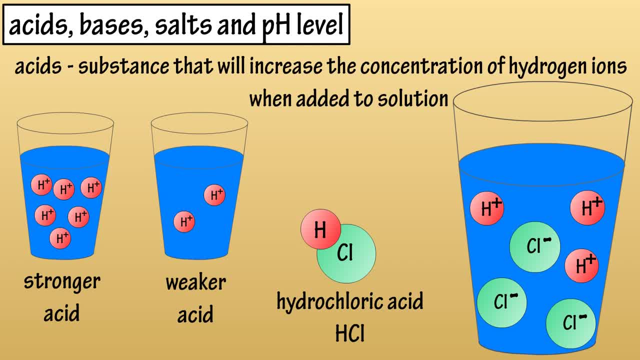 chlorine ions and positive hydrogen ions. Hydrochloric acid is a strong acid as it completely disassociates in water. Now for bases. Bases are essentially the opposites of acids, in that they shift the hydrogen ion to the negative hydrogen ion. So when you add a solution or water, you 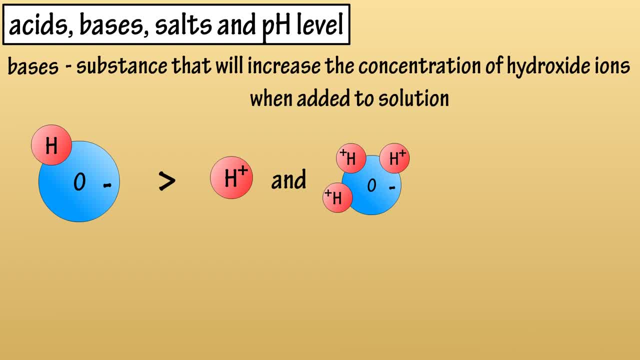 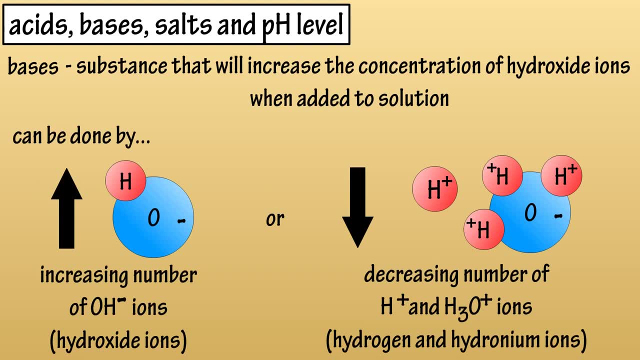 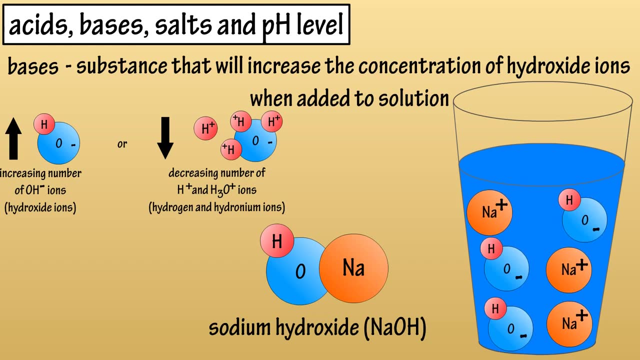 will have a balance of hydrogen ions, Hydrochloric acid, hydrogen ions, hydrogen ions and hydrogen ions. This can be done by increasing the number of hydrogen ions or decreasing the number of hydrogen ions. For instance, sodium hydroxide or NaOH will break down or disassociate into positive Na ions. 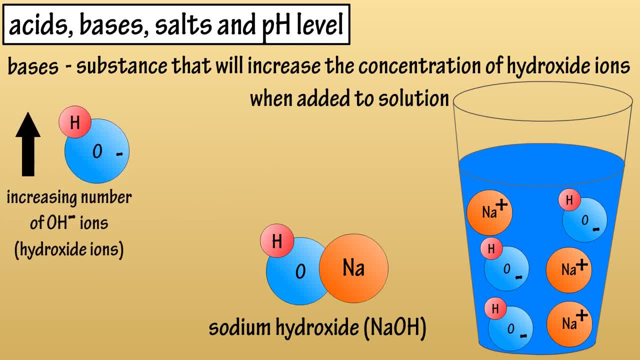 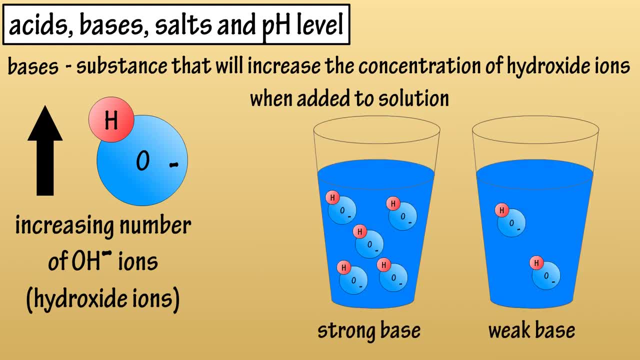 and negative OH ions. So the balance has shifted in favor of the negative hydroxide ions, meaning sodium hydroxide is a base. Bases can also be strong or weak, depending on how well they break apart. Sodium hydroxide is a strong base. This 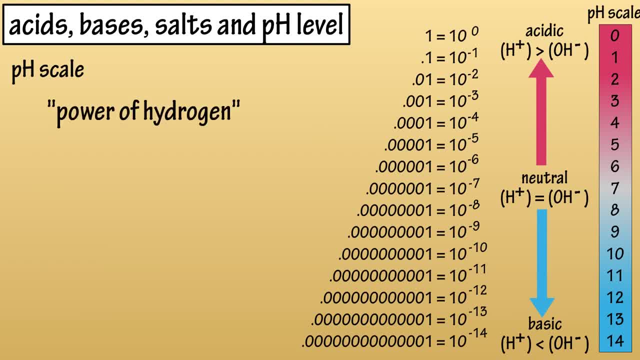 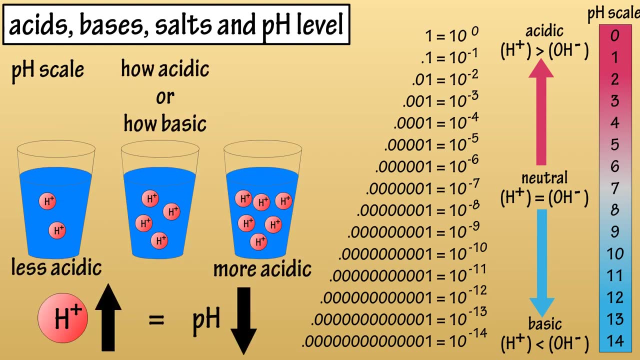 brings us next to the pH scale, which is basically an abbreviation for the phrase power of hydrogen. So the pH scale measures the concentration of hydrogen ions of a solution, or it measures how acidic or basic a substance is. As the amount of positive hydrogen ions increases, the pH goes down. 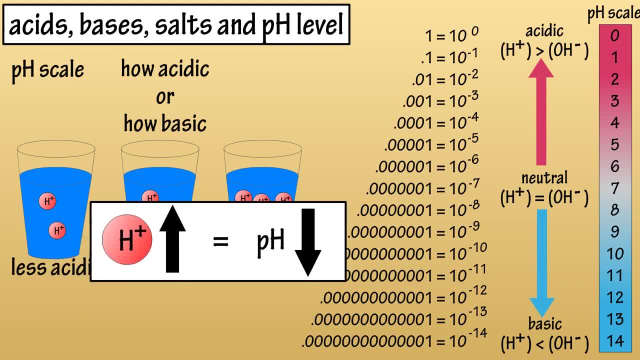 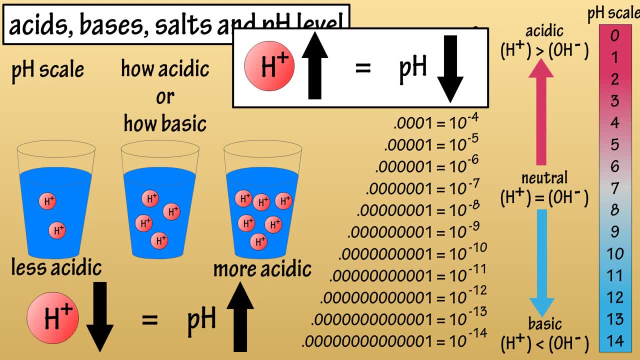 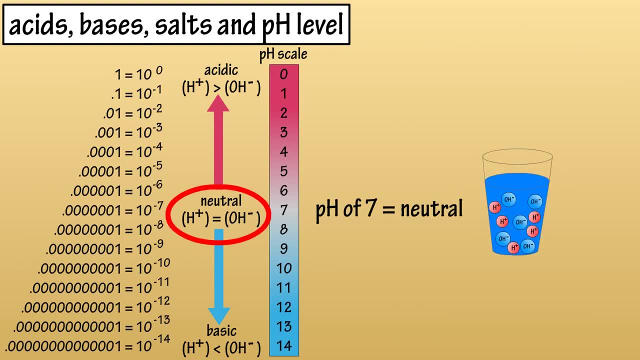 and the solution becomes more acidic. As the amount of positive hydrogen ions decreases, the pH goes up and the solution becomes more basic. On a pH scale, a pH of 7 means the solution is neutral, or the number of positive hydrogen ions equals the number of negative hydroxide. 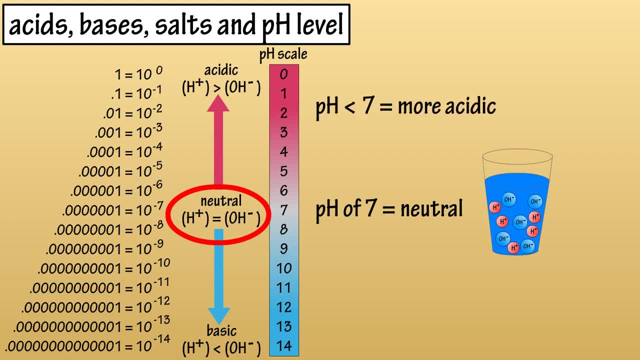 or OH ions. A pH of less than 7 means the solution is more acidic or more hydrogen ions than hydroxide ions, and a pH of greater than 7 means the solution is more basic or more hydroxide ions than hydrogen ions On the scale hydrochloric acid, which we mentioned earlier and is produced in the stomach. 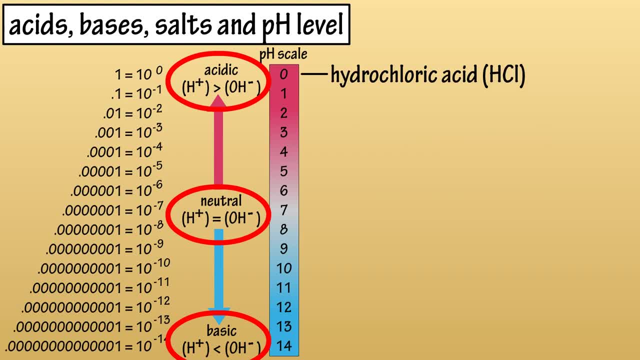 is at the most acidic end, having a pH of 0., Vinegar has a pH of 3,, coffee has a pH of 5, and pure water has a pH of 7, making it neutral On the opposite end, sodium hydroxide, which we 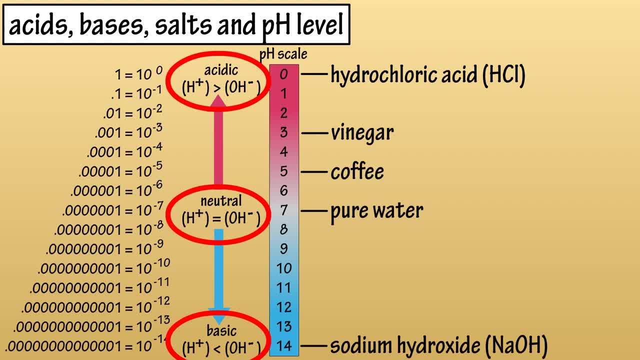 mentioned earlier, is at the most basic or alkaline end, having a pH of 14.. Ammonia has a pH of about 11, and baking soda has a pH of between 8 and 9.. Now we can look at salts. A salt is a chemical. 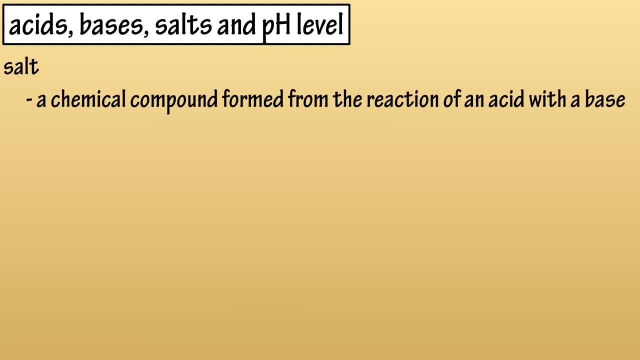 compound formed from the reaction of an acid with a base, So hydrochloric acid. HCl can interact with sodium hydroxide, NaOH, a base, and form sodium chloride, NaCl and water. H2O Salts break apart or disassociate in a solution of water to form positive and negative. 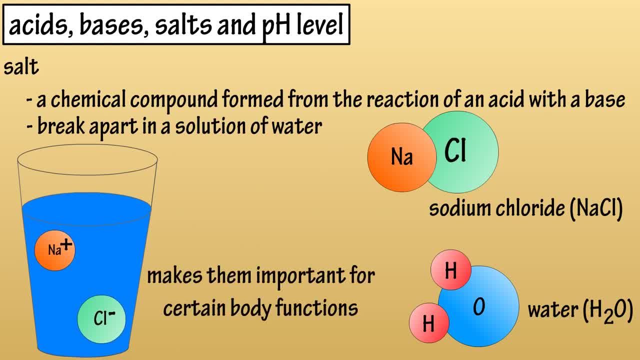 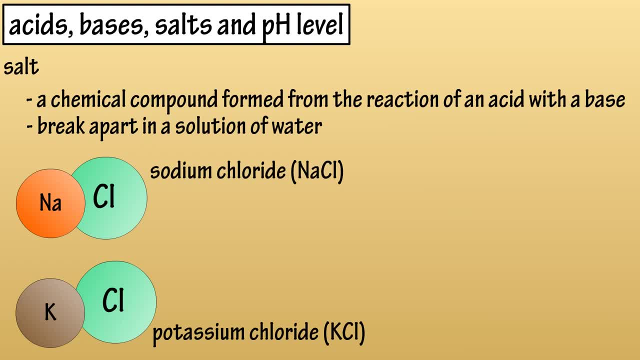 ions, which make them important for certain body functions. There are many different salts that are important in the body, such as sodium chloride or NaCl, and potassium chloride or KCl. These salts are often most effective as charged ions or atoms in solution, as the positively charged